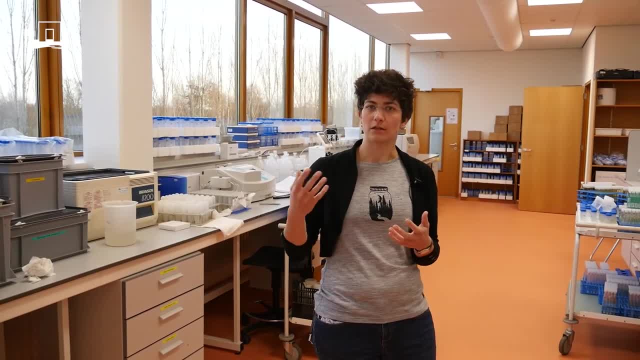 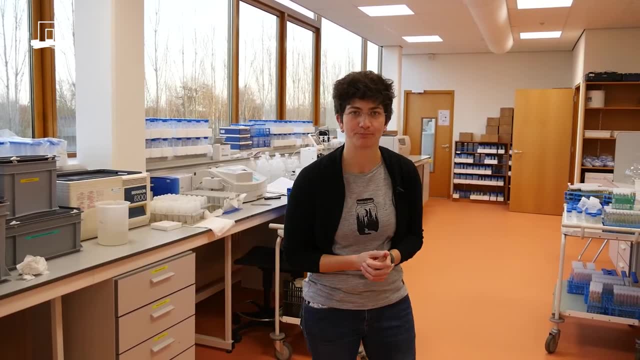 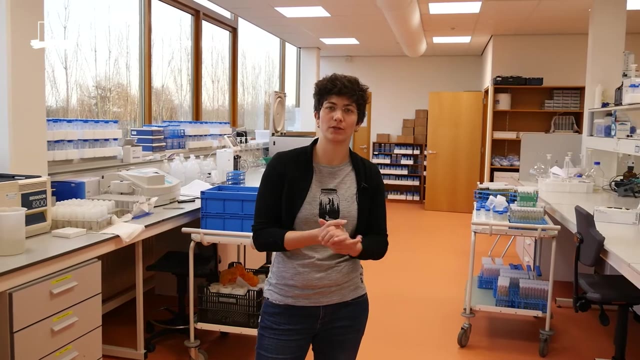 we do extractions or destructions to take the elements in the soils into solution, and then we can analyze with different analytical techniques, And this is happening in this lab basically. So we have here different equipment like centrifuges, water baths, a microwave to destruct samples, And what we also have here is a very special machine. That's the. 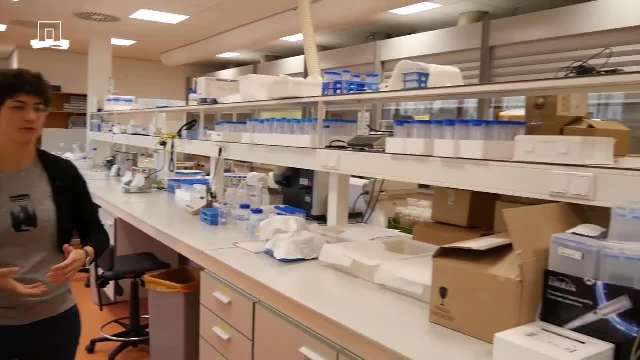 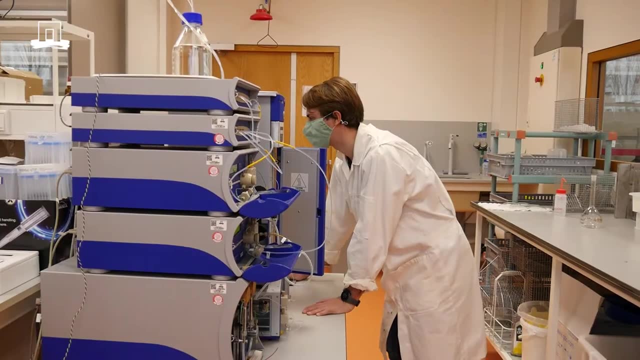 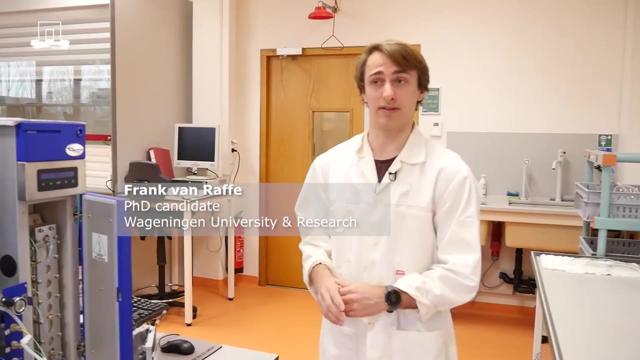 AF4 here in the beginning of the room And I'll give the word to Frank, who will tell you a bit about the machine and what he's using it for in his PhD research. My research is on the contamination potential of landfills And one aspect that's very important in this research. 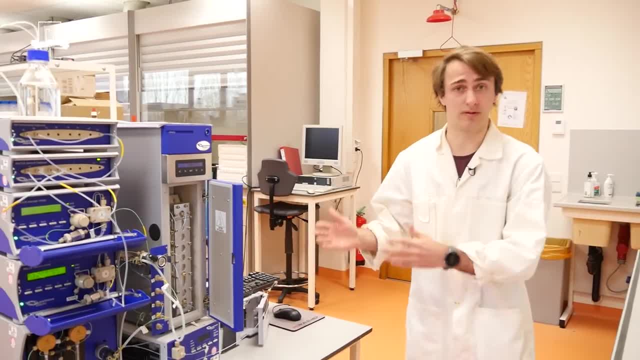 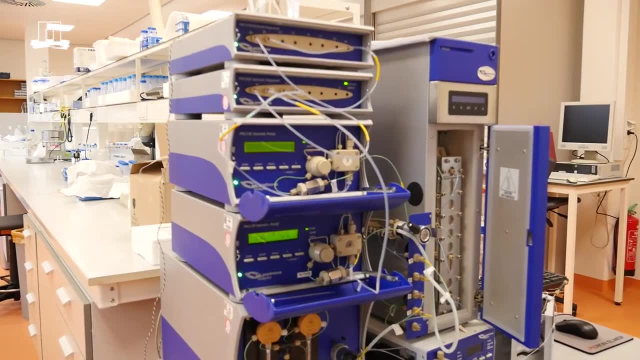 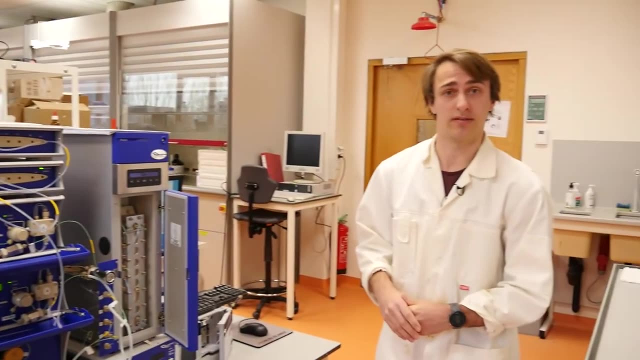 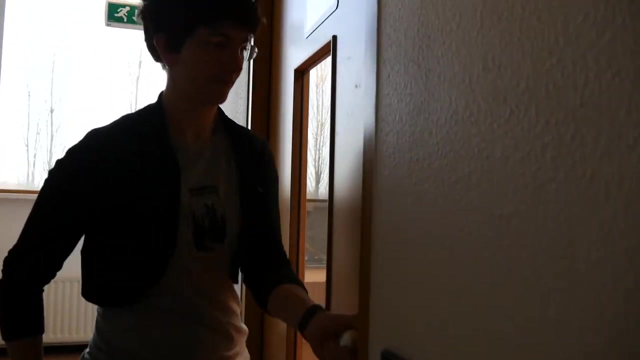 is how contaminants are transported through the soil. This device, the AF4,, helps me in this respect, Because what this device does is that it separates particles and compounds based on their size, And the size is closely related to the transport rate through the soil. So here we're now in the lab where we 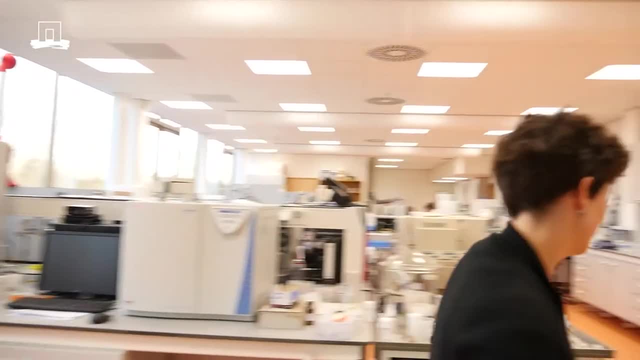 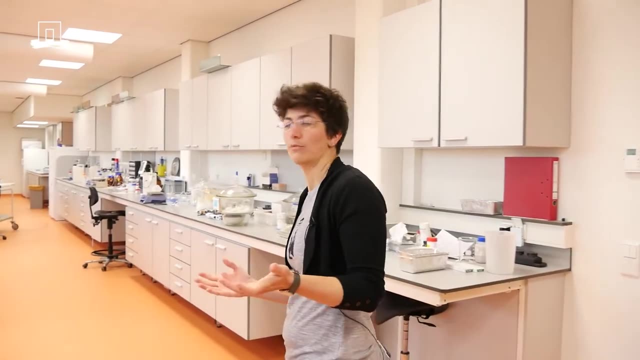 do the chemical analysis. So here we're now in the lab where we do the chemical analysis of our samples. These were soil samples, plant samples or water samples, which we now analyze for the chemical composition here, And we have different equipment to do so. So we have 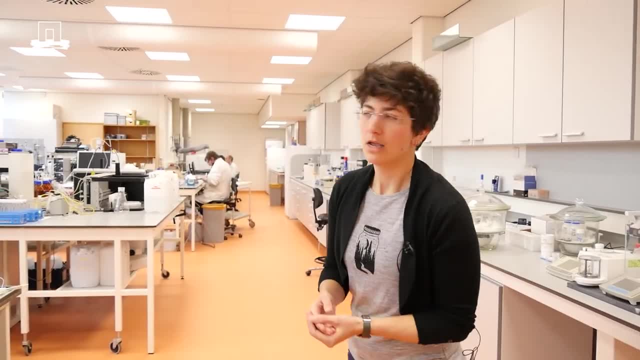 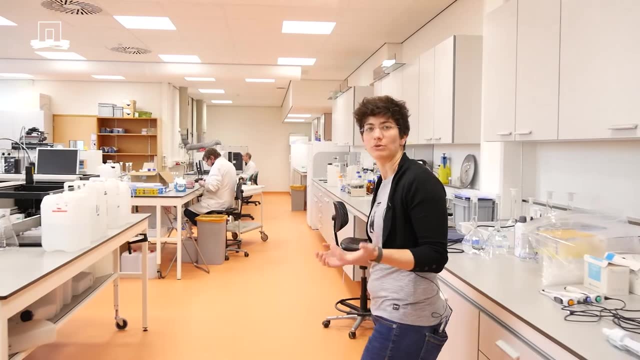 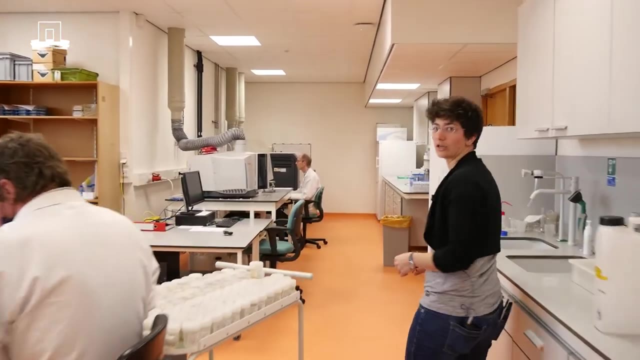 elemental analyzers to determine carbon or nitrogen, different segmented flow analyzers which are optimised for nutrient analysis, And in the backend of the room we have ICP, OES and ICP MS instruments. These are located over there And I'll here give the word to Frank. 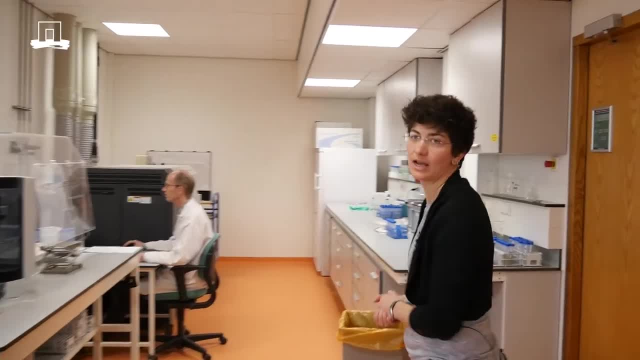 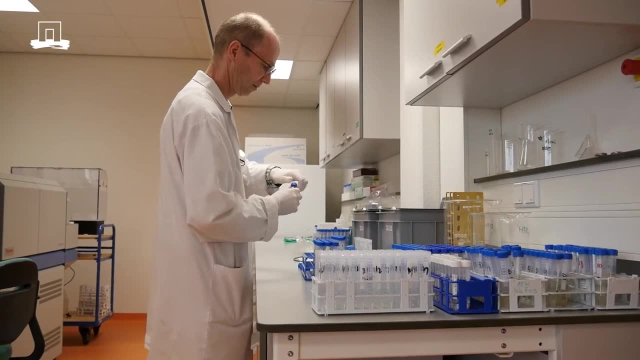 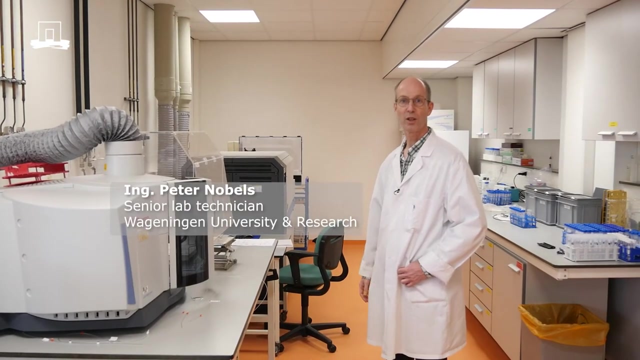 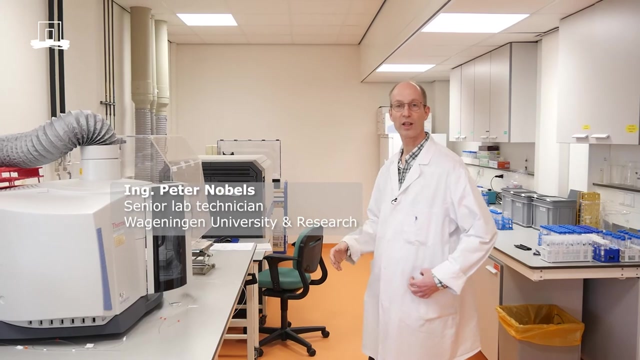 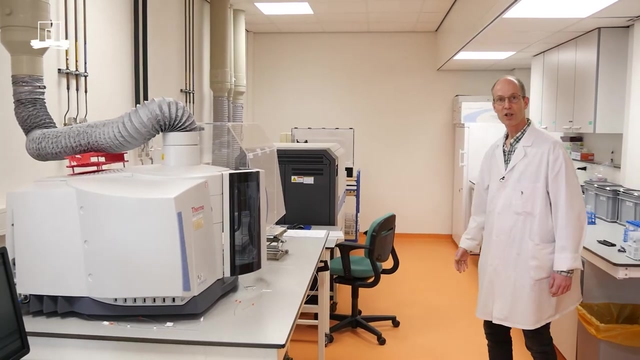 to Peter, who is a senior lab analyst in our lab and ICP MS specialist. okay, so there are extracts made or digests made from soil or plant material, or there are waters, and that we are able to measure elements inside these extracts, digests or waters. here we have an ICP OES and we have an ICP MS and